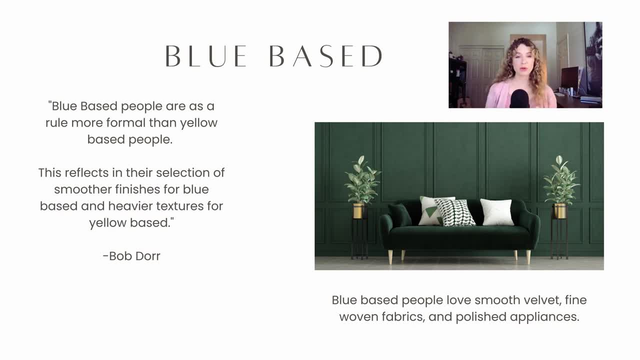 heavier textures for yellow base people. So this is something that Bob Dorn found in his research when he was studying the differences and the preferences between blue and yellow base people. He found that blue base people love smooth, velvet, fine woven fabrics, polished appliances. 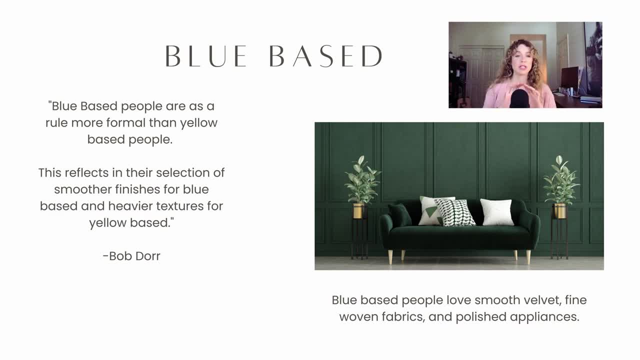 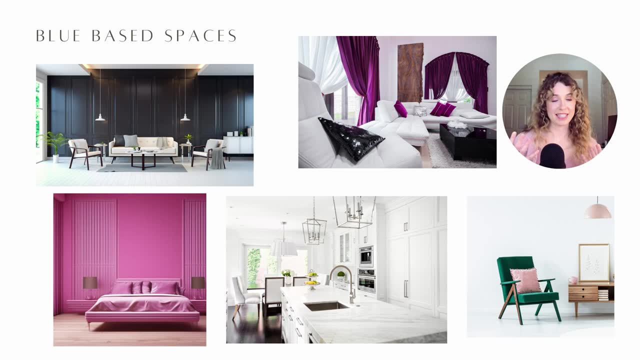 things that have been polished, smoothed, dyed, things like that. I'm going to show you some spaces here. All of these spaces are blue based spaces. All of the whites that you see here are white white. It's a very modern thing to put white white in your kitchen. It looks very clean. 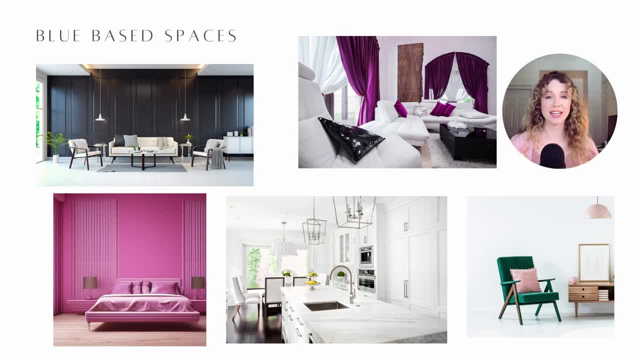 and fresh, And that is a blue base thing to do actually. And the appliances there are all smooth, stainless steel. That is also a blue base thing. The pink and the purple here, those are blue based. The green underneath me, that is blue based And, as you can see, everything is really. 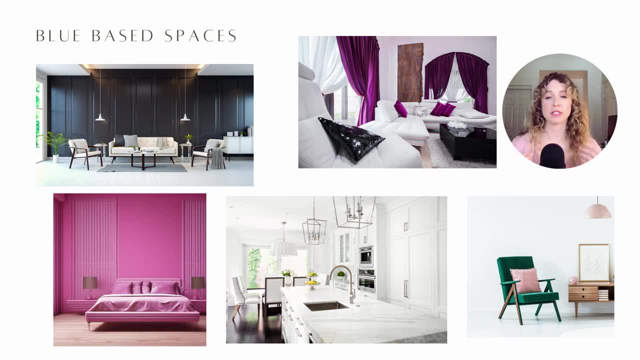 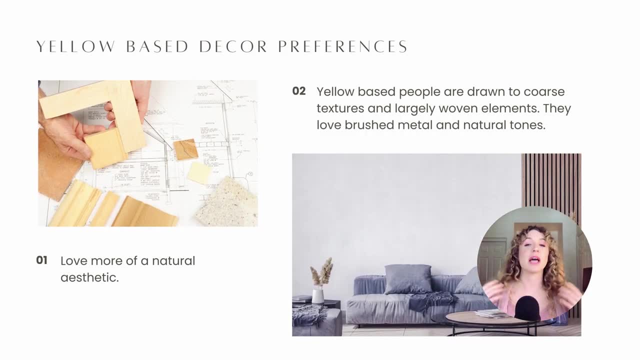 smooth, polished, finely woven fabrics, smooth velvets. Yellow base people prefer more of a natural aesthetic And this is because they love those heavier textures. Like Bob Dorn said, yellow base people are drawn to coarse textures, largely woven elements. They love brushed metal. 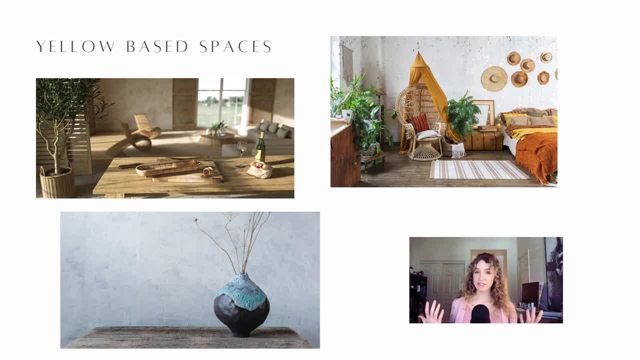 natural tones. Let me show you some examples. Fun fact: blue base people are more willing to live in yellow base spaces than yellow base people are willing to live in blue base spaces, And this is because yellow base spaces tend to mirror nature more. Think like these natural wood tones. the 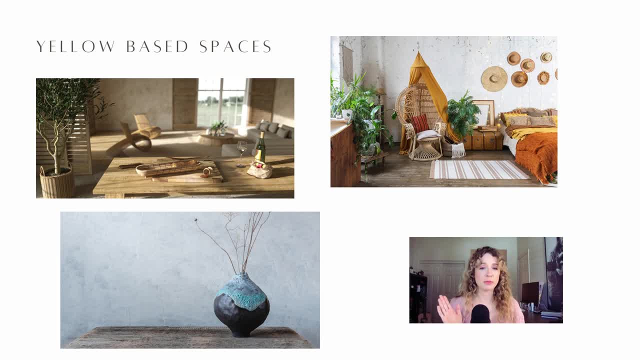 blue here, the tones above me in that bedroom, the oranges and the yellows you know, reminds you of autumn. None of it's really that manufactured color. It's more of the colors that you would see on a walk in the woods right. Even this blue to my left here that is a very yellow based. 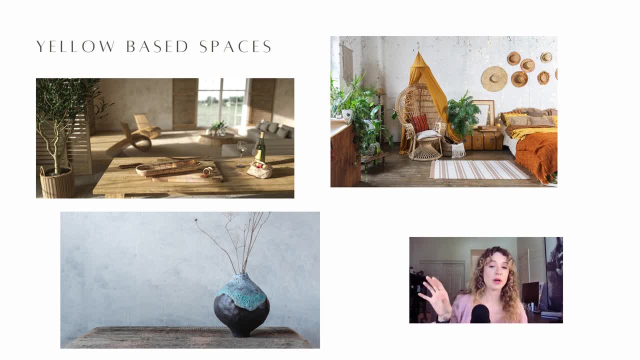 situation with the coarse wood and then the blue stone that is more textured Yellow base. people love textures and natural aesthetic. This actually goes into the jewelry that they like as well. They also like natural stones and natural, not really finely polished, but more of like that natural metal When choosing wood for. 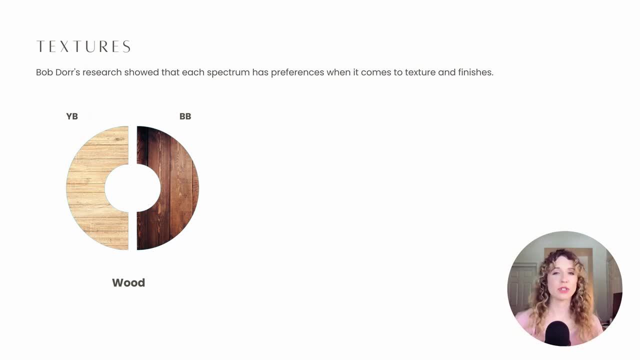 your home. as a yellow base person, you're probably drawn more to rustic woods, bamboo or wood. that is in its natural form. It's natural aesthetic. It just got chopped, It just got axed down and it got cut. but it didn't necessarily get cut, It just got cut. It just got cut. It just got cut. 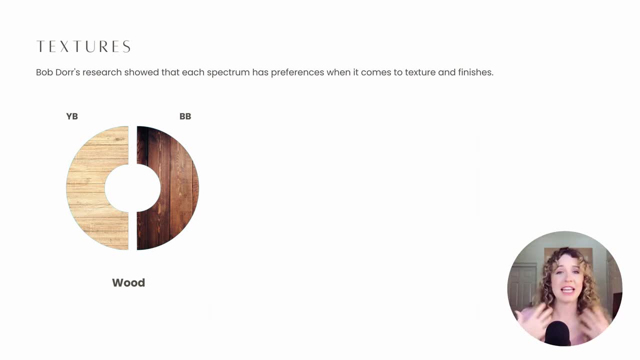 I actually love this look too, As a blue base person- a natural wood table, love it. as blue based person, though, On the other hand, usually likes more stained woods, wood that has been polished, cherry mahogany, Um think, like these darker woods would that has, you know, had a. 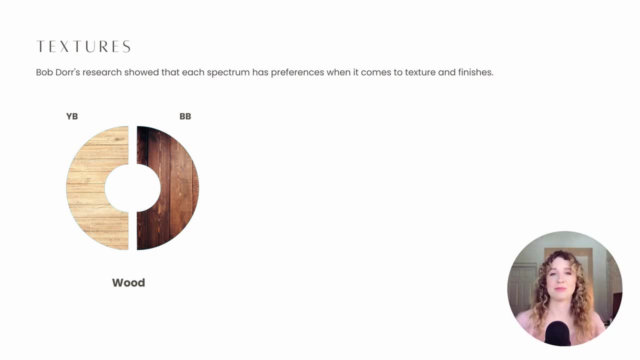 little love, put in and and look really nice and polished. yellow based people love brushed metals, while blue based people love smoothly polished wood, Stainless steel type shiny metal. but yellow based people don't care if it's shiny or not. They would, like you know, iron more than stainless steel, For example. 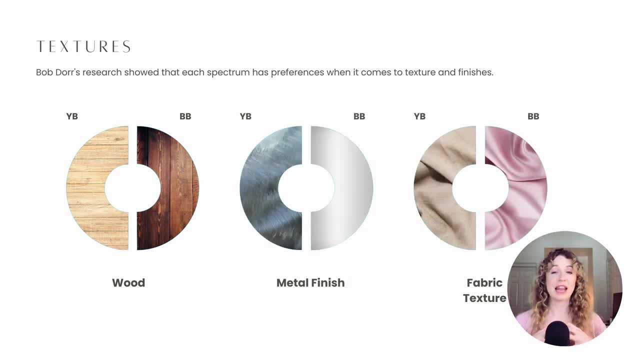 like I said before, yellow based people love that heavy woven fabrics like raw silk, crushed velvets, where blue based people love smooth silk, smooth velvet, smooth leather. even So, a yellow based person is going to like that rougher leather that looks like it just. 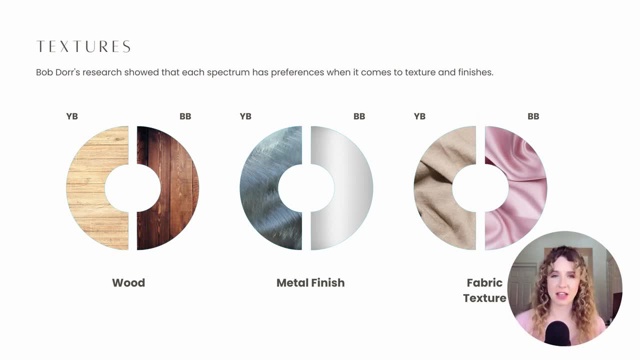 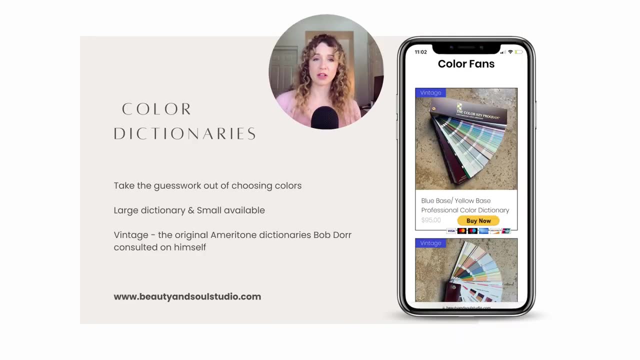 got made, but blue-based people are going to like maybe the synthetic leather more because it's smoother. If you still have a hard time figuring out the difference between blue and yellow-based colors, have no fear, We are here. We have some vintage color fans that Bob Dore consulted on himself. 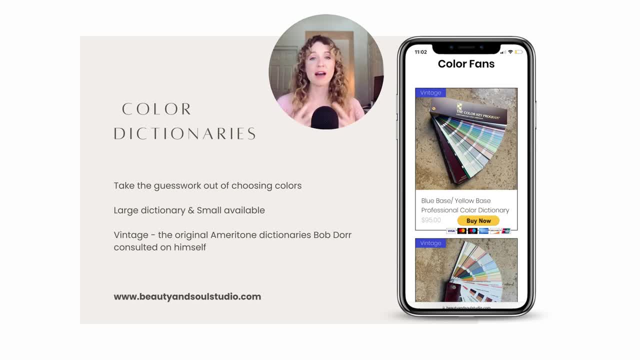 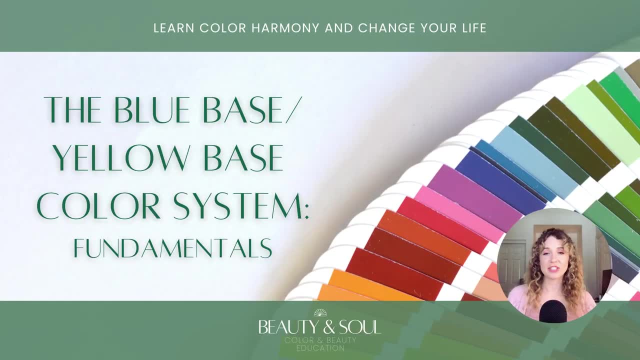 These are the original Ameritone color fans. We have the last ones in the world, So if you want to get them before they sell out, go to our website. We have officially launched the blue-based, yellow-based color system fundamentals course. It is officially: live In this fundamentals course. 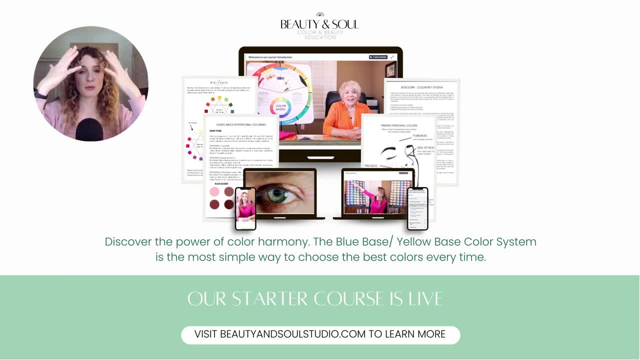 we go over how to figure out your perfect colors, to wear your personal coloring and how to analyze your colors yourself. We also go into tons of fascinating research and stories about this system. That's all I have for you today. Thank you so much for watching and I'll see you.